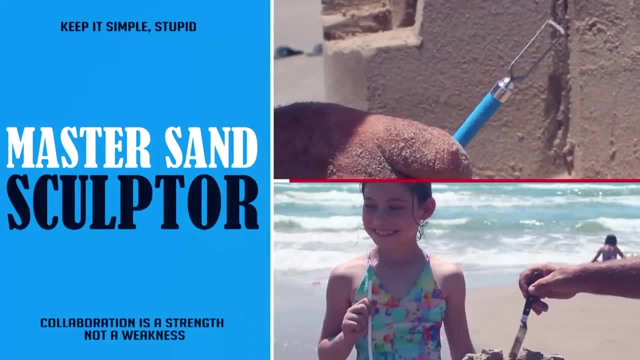 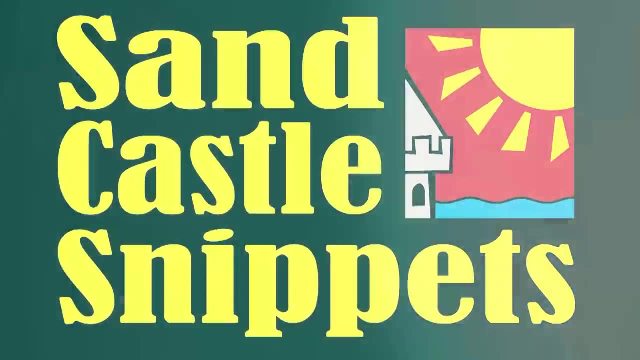 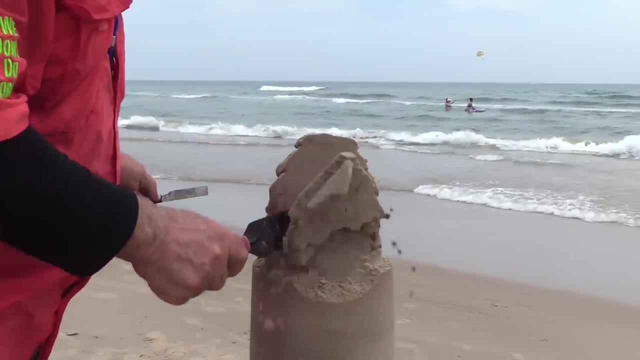 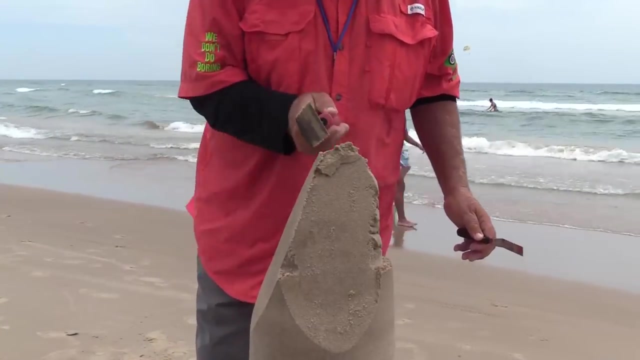 So welcome back to me, Andy Hancock. Sandcastle Snippets, simple tools on the beach, and what we're doing is we're just using the big spatula, because we found that if you use the big one, you can do a roof very, very quickly. I always start with a square roof. I just like to know that it's actually. 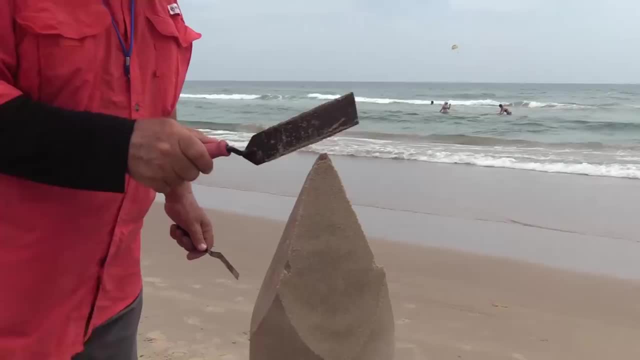 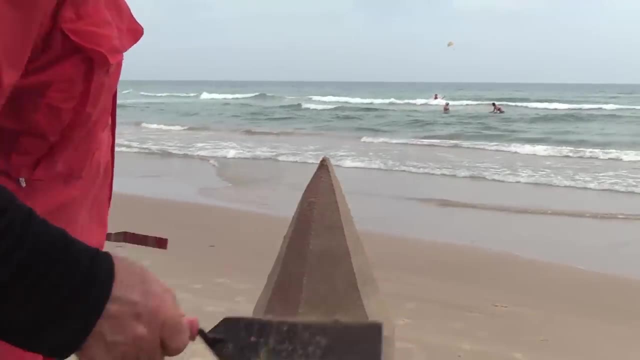 looking straight up and down and start with the square, square pyramid and then just take the corners off. So if you take the corners off, you can then make it look like a pencil- we like pencils- and once you've done that, you can see whether it's straight and just. it just makes it easier to do. 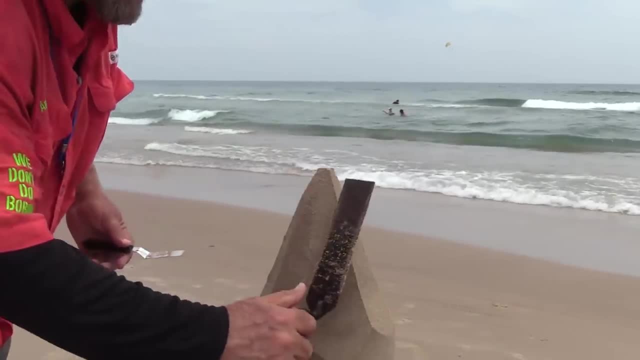 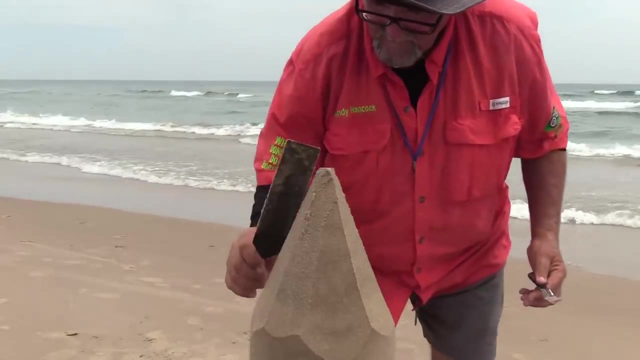 and then get it nice and round. So the way to get it actually smooth is to use your big spatula and just go around and just gently clean off those lines and you can get it to look like a perfect pencil. So it's nice and round on the end and that's it. It's very fast with the big spatula. 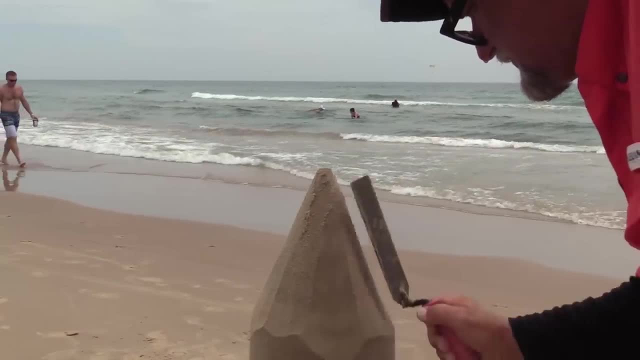 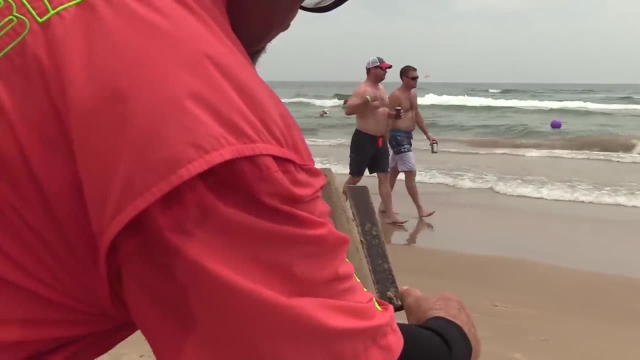 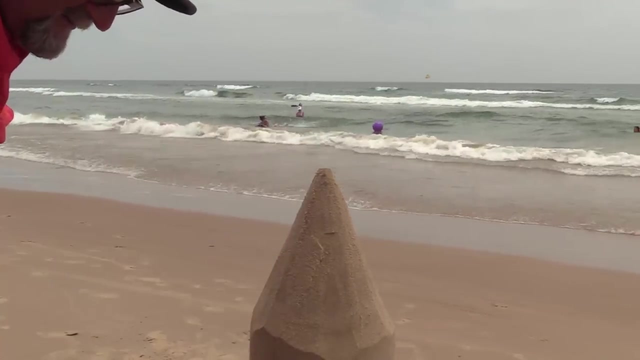 it has such a stiff blade that it's very easy to keep the edges flat. and oh, this is two chaps again, right, and they've got beer and you didn't bring me one. oh, what a shame. never mind, I probably didn't notice at the time because I was too busy. Anyway, so you can do that, moving swiftly on, do that and 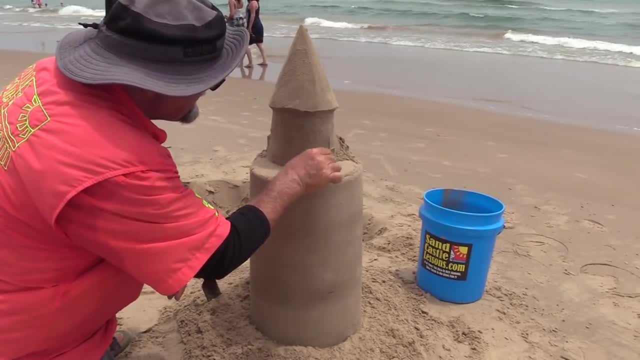 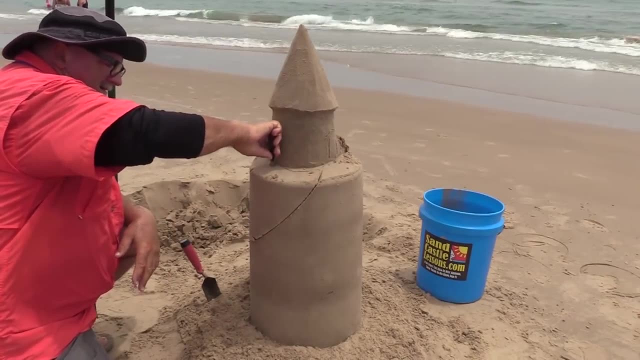 then you can see that we've jumped a bit here because apparently the shot I made wasn't it the eave, that's the bit that sticks out of the roof in a minute. So when we're going to do the stairs we're back to our small spatula and we can just chop a big chunk out like that and another. 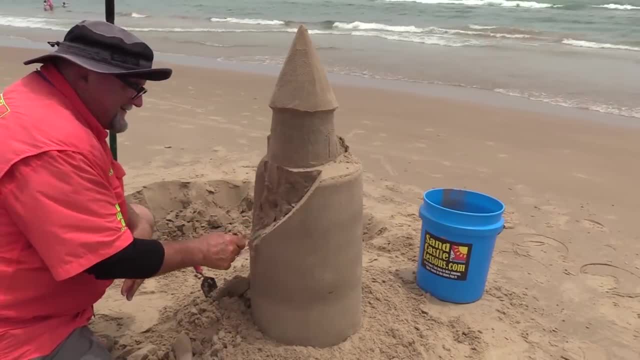 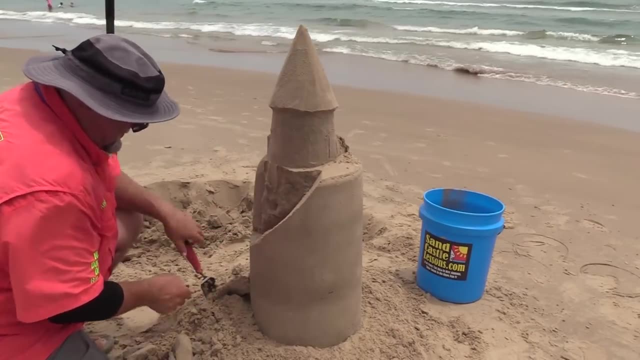 big chunk and just pull it away. We don't care whether it looks broken on the side, because we're going to make that into stones later or we can smooth it off, it doesn't matter. So the important thing is the bucket was pushed over to one side, so you've got this big step on one side and the 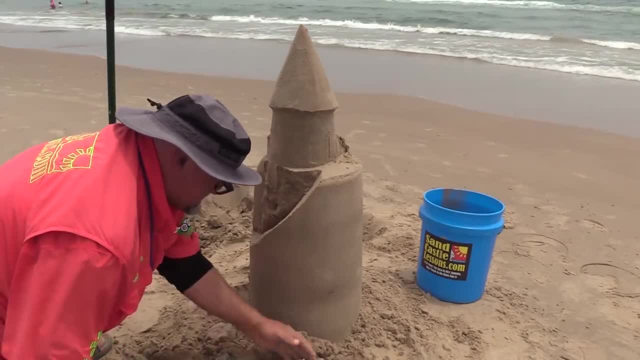 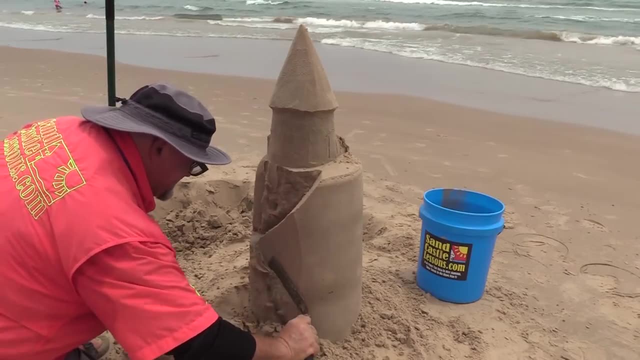 step gives you enough room for the stairs. The other thing we're doing today is showing you how to reuse the sand that you carve off, because a lot of people don't know how to reuse the sand. People throw it behind them, which is seems like a bit of a waste, and we like to recycle ours and 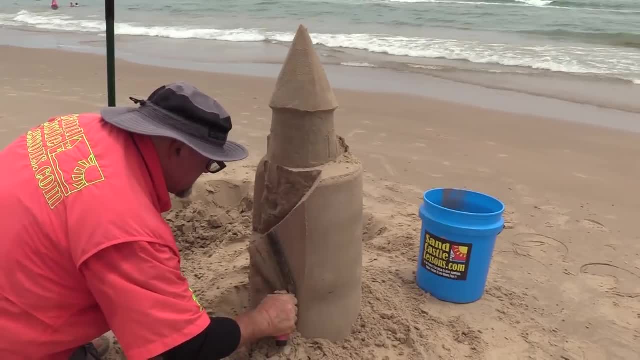 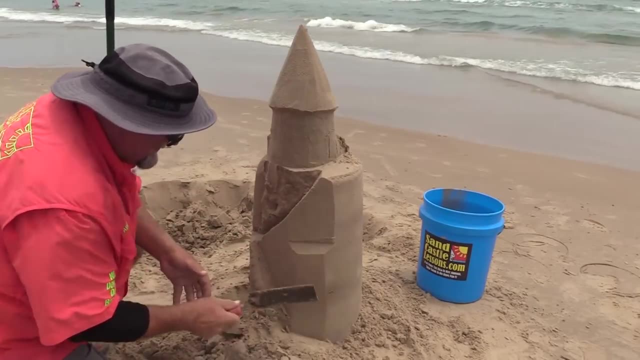 use it for other things, So. but what we're doing is making a return on our sandcastle staircase. So we do one stair that comes down from the top, and then we stop on a balcony or make a little ledge and then we have another set of steps going the other way down to the floor, and you can see we're. 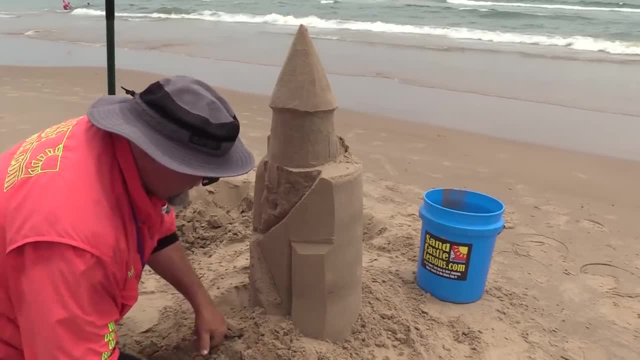 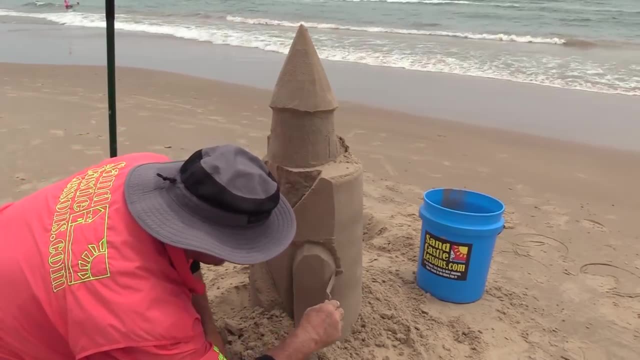 going to put a bit of a doorway in here. so we're doing that. So you can see that I can. I swap, I switch between the big spatula and the little spatula, So I'm going to put a little bit of space in here because it's just, you've got a bit more control and and it enables you to get into. 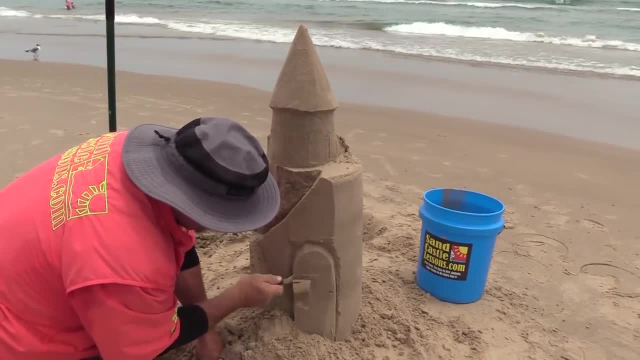 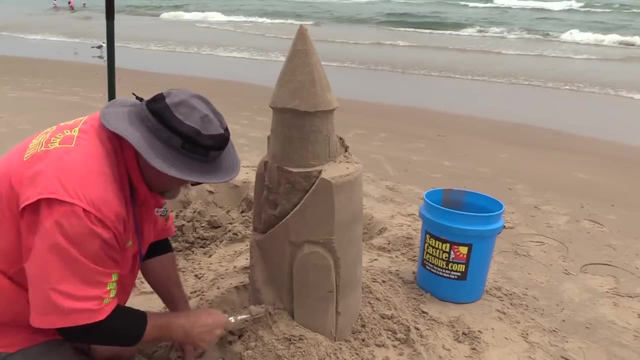 smaller spaces and that sort of thing. so that's why. but the two spatulas are going to give you the ability to do any amount of detail. I mean quite staggering really. So, as I say, there's the top stairs, the bottom stairs, and then what we've done here is we've, we're going to make a little. 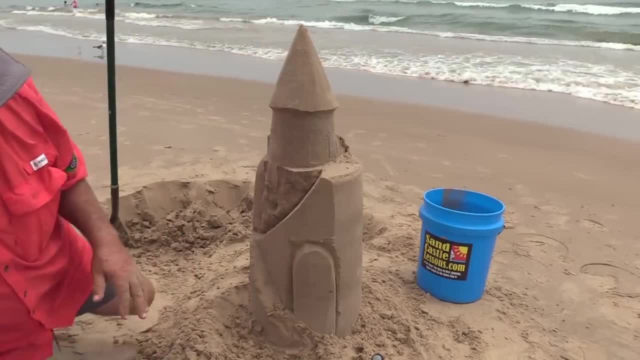 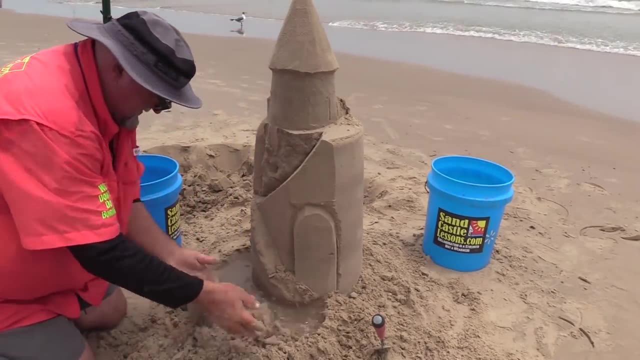 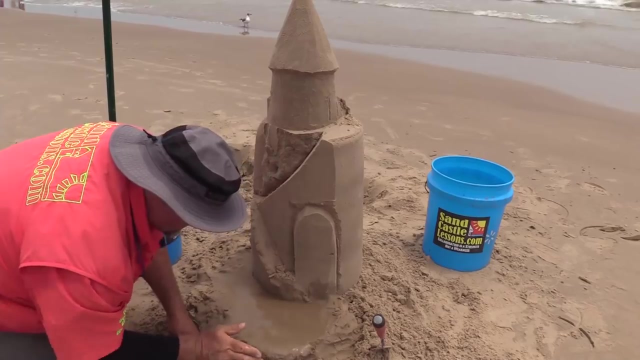 moat again. we like making little moats, um and uh. so we make a little moat, we fill it for the water, and then what we do is we fill it for the water and then we fill it for the water, fold the sand in very gently into our little moat and then that makes us a nice, solid pad of sand. 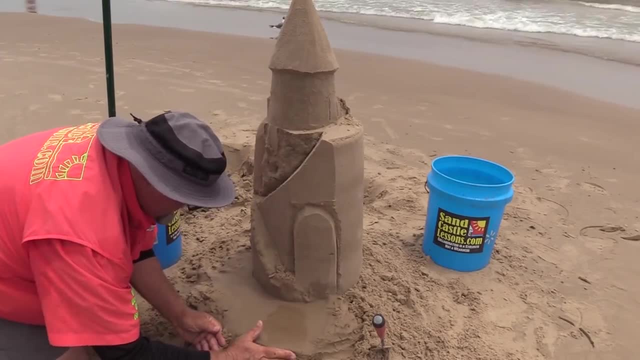 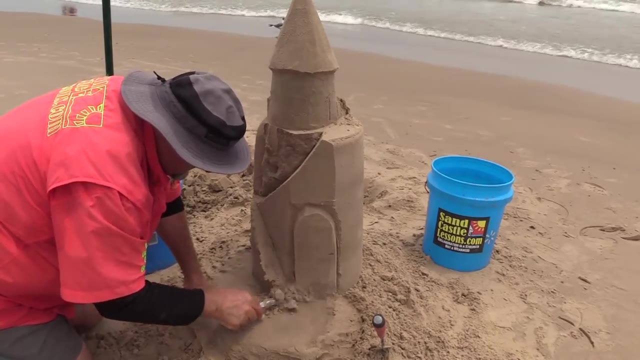 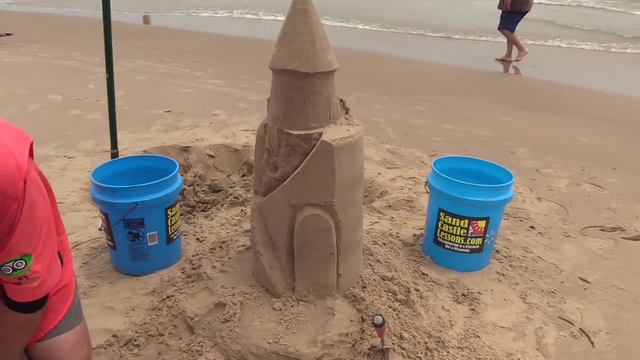 which then means we can join the stairs more effectively. sometimes you run in a room on a cylinder, you run in a room for stairs on the outside, so it makes it a nice even deal like that. and uh, there we go, so we've, we've done that, so we bring it down, and then, uh, what we're going to do? 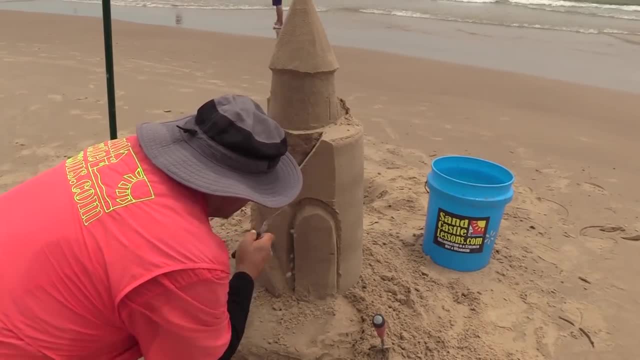 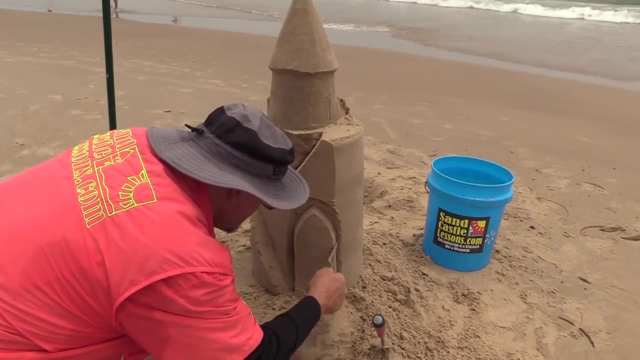 now is scrape off the stairs and and just roll it down, and then we're going to do a little bit of redo this doorway a bit and uh, I like sort of arch church doorways, so I like to do them like church doorways, old-fashioned church doorways. so do that, and then we can just screed it off and make. 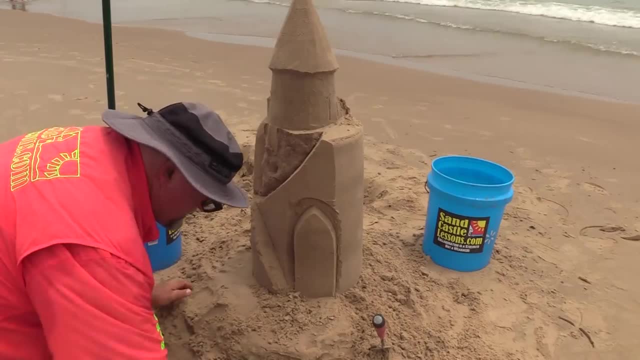 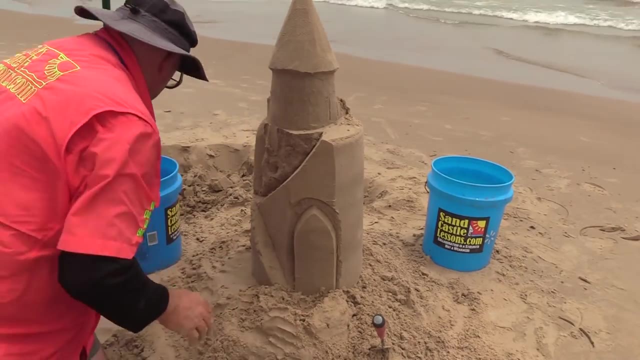 it look better. um, and then we again, we're going to use our sand. oh, put a bit more sand up here, because what we decided to do now is that the stairs still don't quite reach, um, and don't look right. so you again, you make a little little moat, pour your water in and then just fold the sand in. 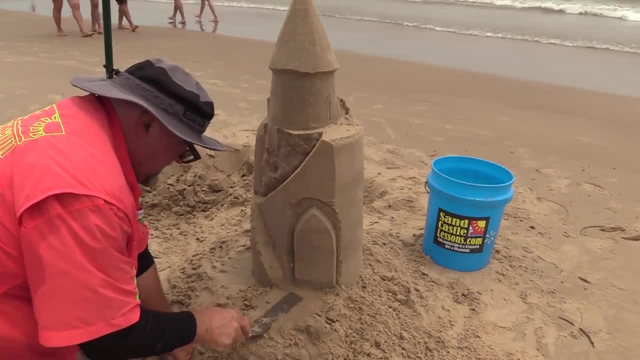 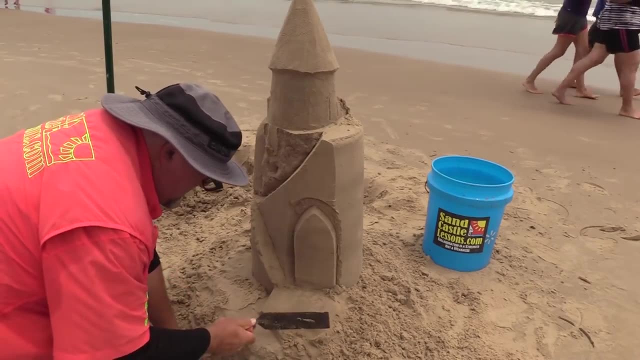 over the top, and if you do that you're going to get a little bit of sand in there, and then you're going to be able to just pat it together with your spatula and make a proper pad where the stairs can come down onto your by the doorway. boom, boom, boom, like that. okay, and then you better flatten. 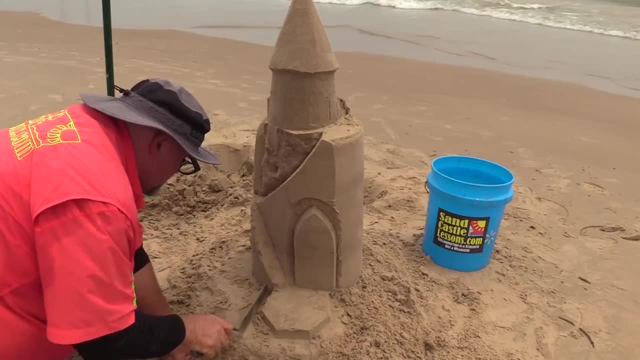 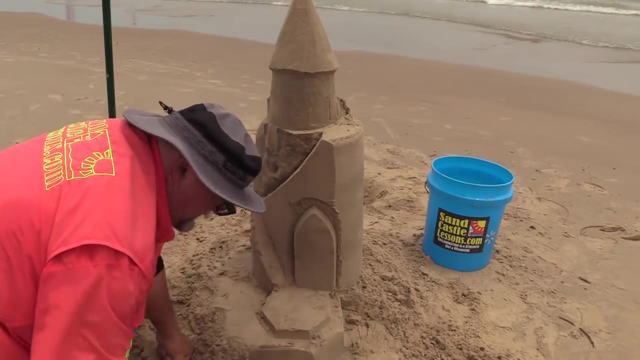 it out and make it right on top. so there you go. um, yeah, and then you can also make the pad that it sits on even bigger so you can copy the shape. if it's a hexagon or an octagon or whatever, you just copy the shape and you can use. you can see how fast. 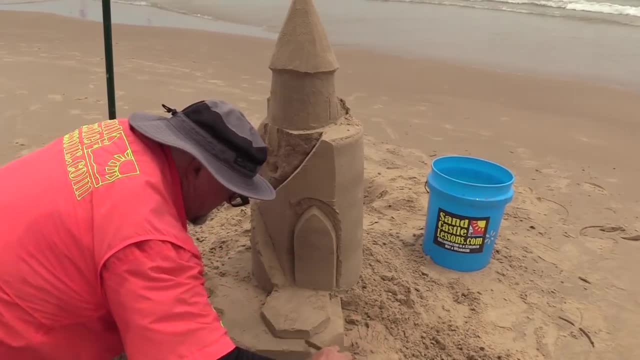 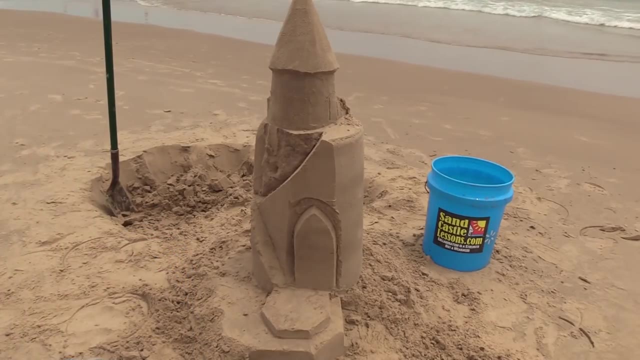 you're moving and people always say this. they always say, well, andy, it's all right for you, you're you've, you know you go, just go so fast. well, speed doesn't come with from anything but experience, and so the more you get out there and practice, the faster you'll get um. you know a lot of young kids. 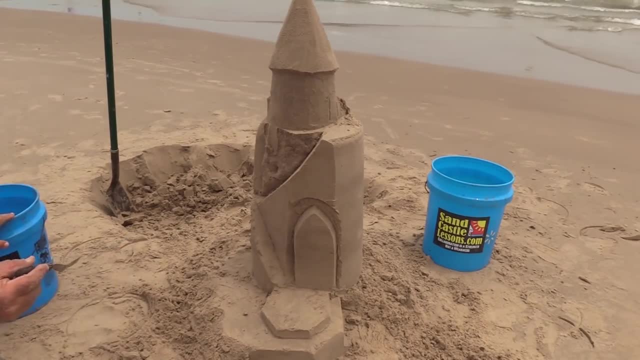 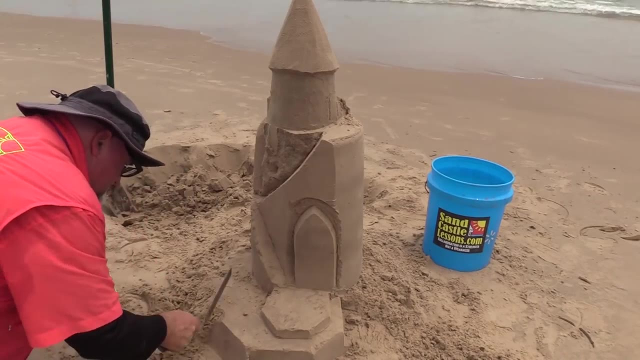 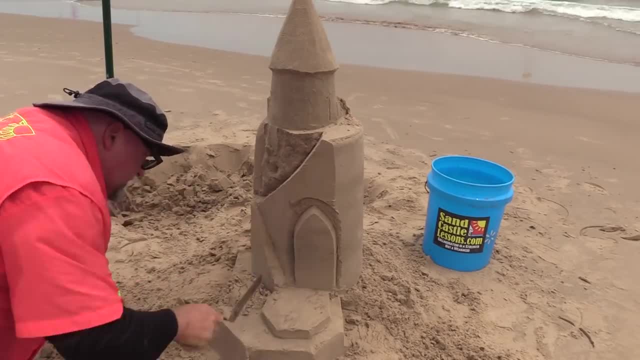 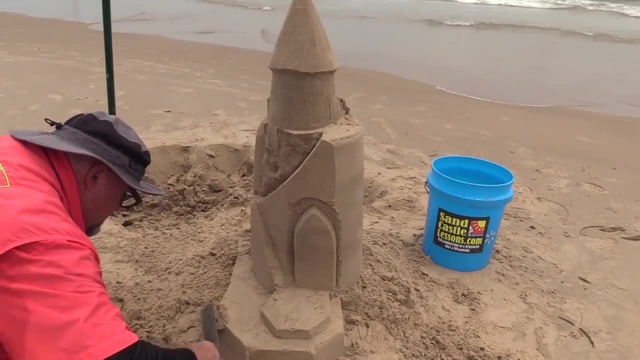 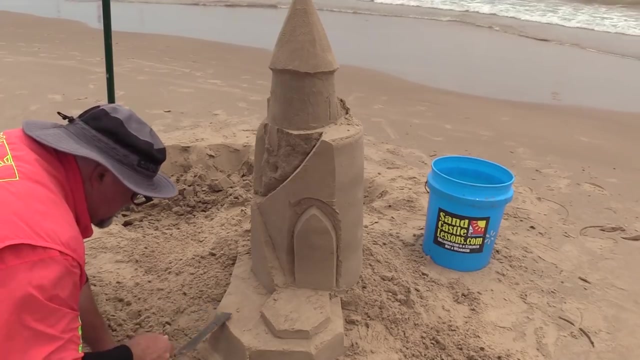 quick. so experience is what makes them quick, makes you quick, not natural ability. um, some people have the ability to see, um see things in perspective quicker, or or um draw things naturally, um, but not many and most people just have to practice quite hard and then they get to learn things and off we go, and that's where speed comes. 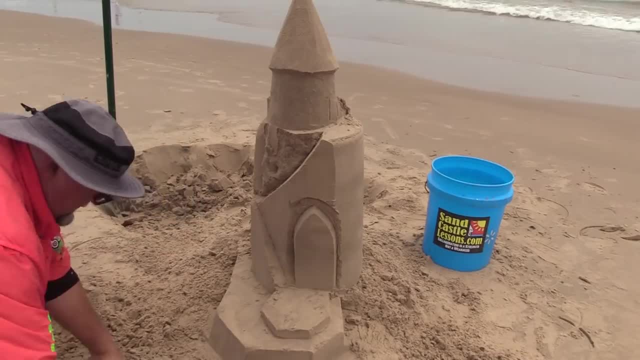 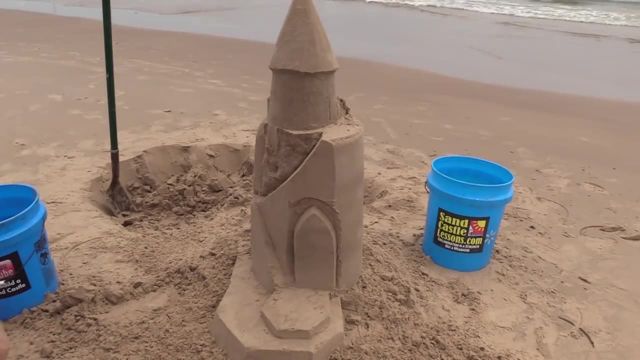 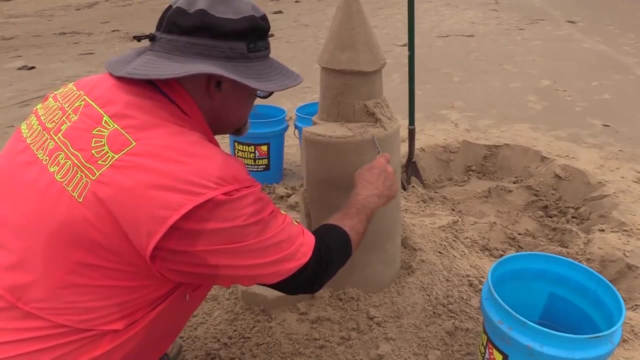 from. i use a chainsaw as well. i'm a chainsaw artist and speed only comes from once. you've practiced a shape again and again, and again and again. you know so, um, that's how it is, but anyway, you're filming like this, yeah, uh, but that's kind of the key, depending on how the character submission. 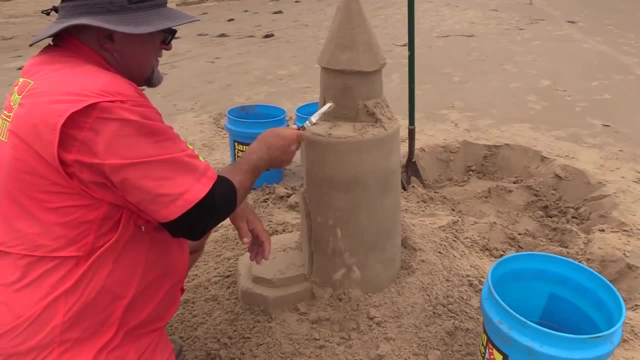 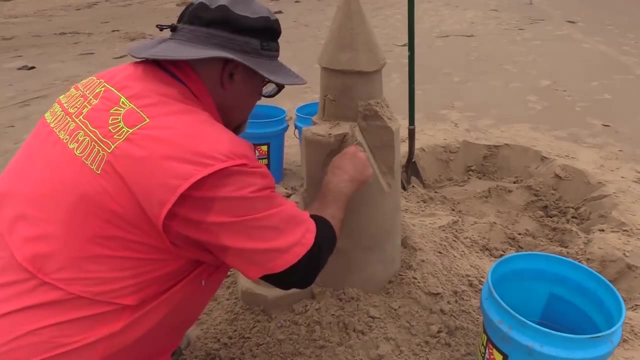 results, i think to me is see the shift mentality. to describe, uh, you need to consider a texture and then know the other characteristics of it. so when you're at this point you know if there's not time for, um, pretty much nobody else to make the shape if you have everybody else in place. 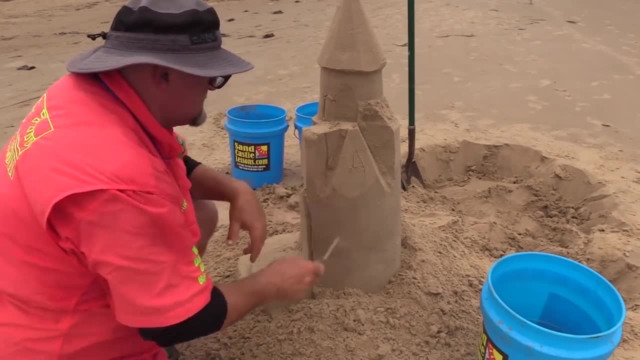 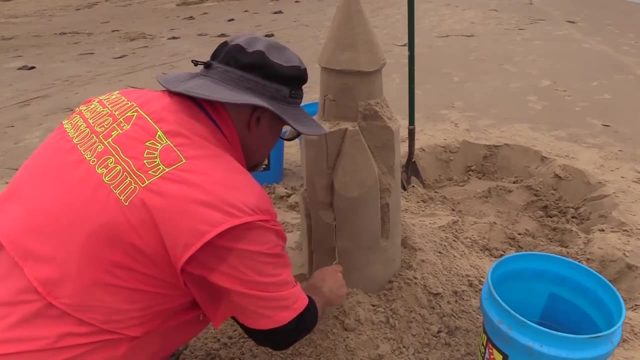 that makes it hard to discover and you need to stop and start living like that. you will notice less times. you will end up better than the people you meet. you will hear more people tell you better, nevermind, And um, you know it wasn't a good spelling day, So, um, so we do that and we go. 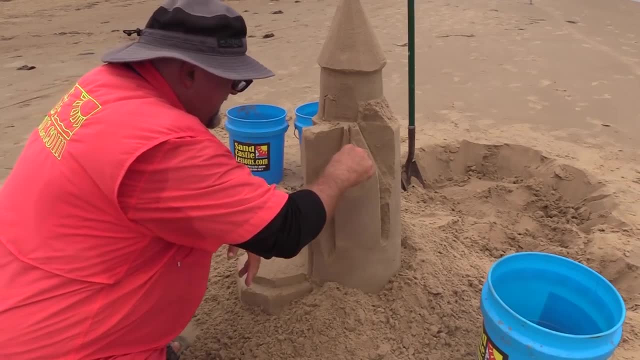 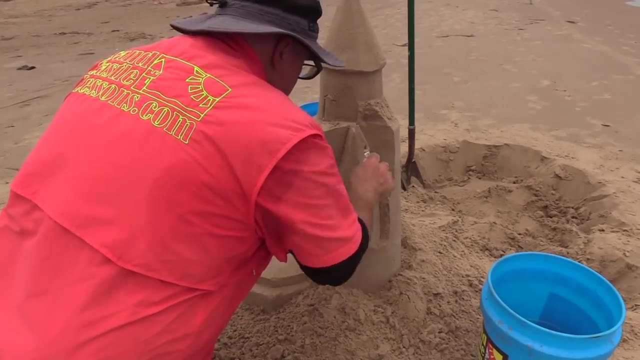 down here like this and just chop it off, And the little spatula gives you so much more control. The big one is good for ripping out big stuff, but, um, the small one is really what you need to master. If you can master this guy, you can make anything. Now, what we missed on the first: 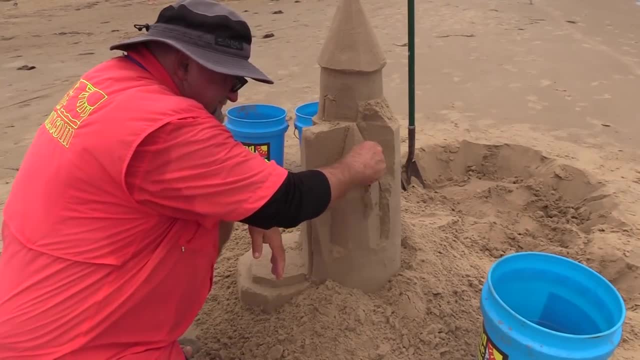 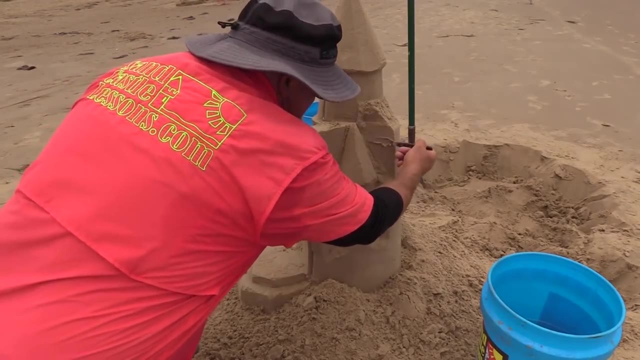 bit was how to put the edge on the castle. So we turn it upright like that and we just scoop it around and you can see it makes the Eve. and the Eve on a castle is the- uh, the edge on the roof. That means the water doesn't fall down onto the wall, It drips straight off onto the floor. 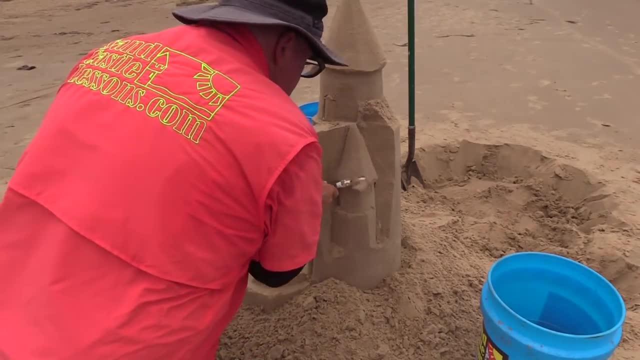 which is much better for your castle, means you. you don't get wet walls, and we don't want them, do we? Especially not in tropical South Texas. So, um, but uh, that's what it's for. It's called. 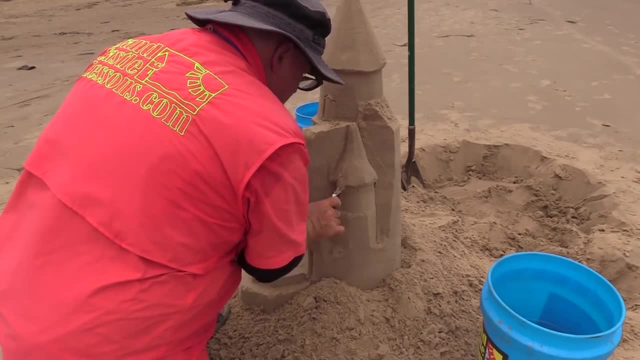 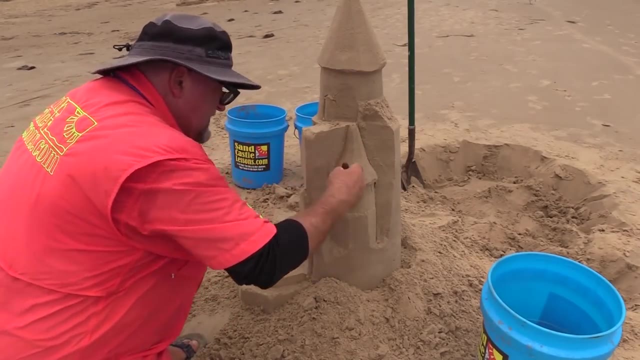 an Eve. in architecture It's probably called something else in America, but that's what it's called in England. So an Eve. and then you make that, and then you can straighten it up with your little spatula and you can make that little tower pop right out And this is called relief carving. 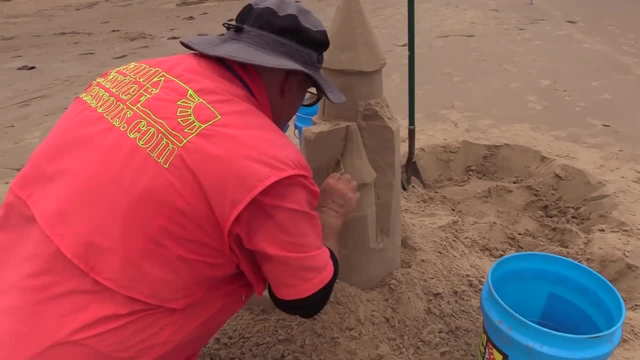 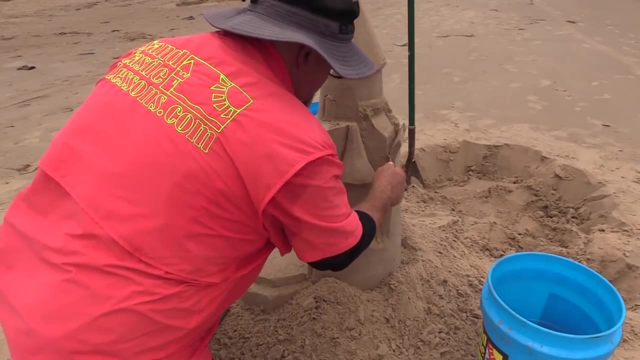 You're relieving the surface, So you're putting one surface on top of another rather than carving it all the way around, which is called in the round carving. So, um, there we go, And if you want another sort of tower, something, very fast, you can just carve like a roof, and like a slope roof, at like 45. 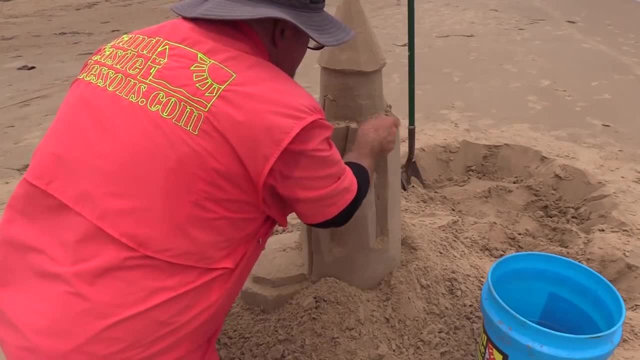 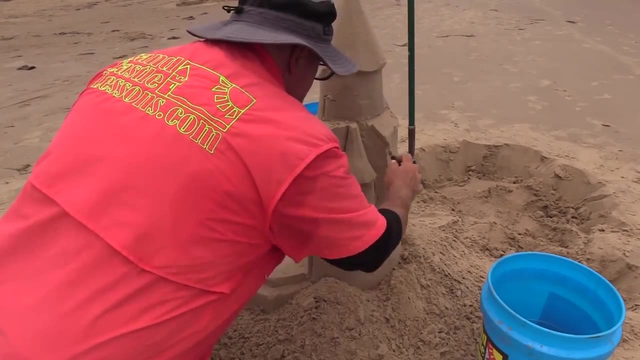 degrees, Okay, And then take that across like that and then cut out the Eve, the little overhang, and then just go straight down using that in step on your spatula. Again, that little cut in bit, um, it's called an in step, So you can just carve like that. And then you can just carve like that. 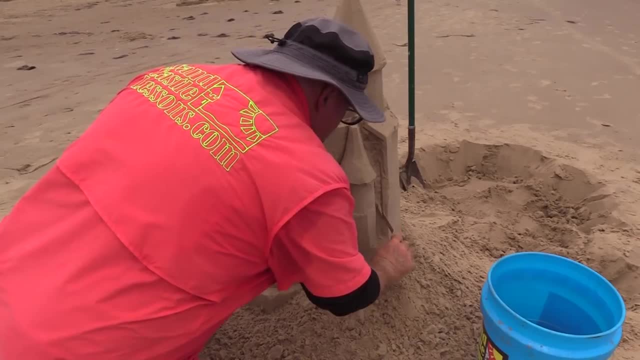 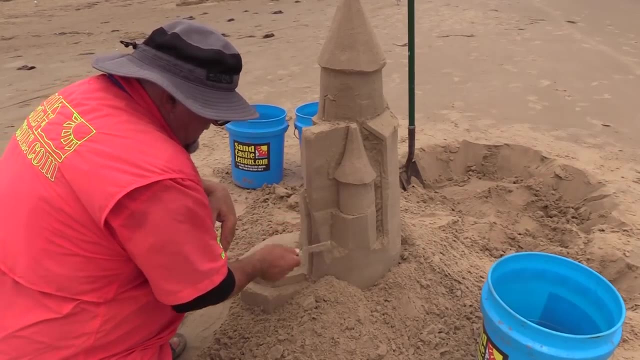 An offset spatula, So we're just using that little offset to cut in this. Now, what I'm doing here is I'm trying to separate the little tower from the, the building next door, And the way to do that is to cut a little line and then just chop out some texture And, um, you can just pick it out with. 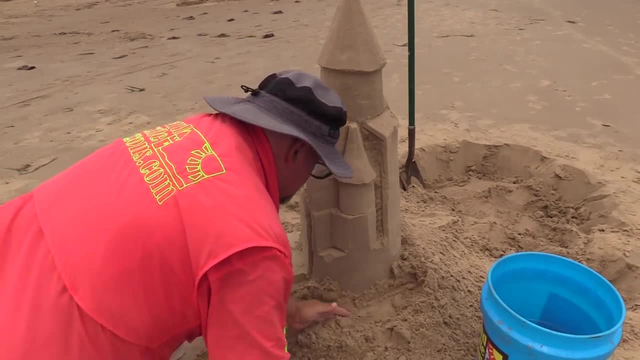 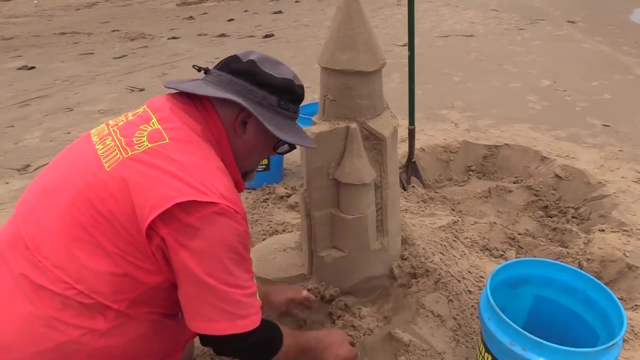 your, with your, with your spatula. Very, very simple, And it means it. you see how it's delineated, or separated, those two buildings, And that's very important as well, because when the shadows catch it it'll look even better. And, um, so we do that, and then we make another little pad. 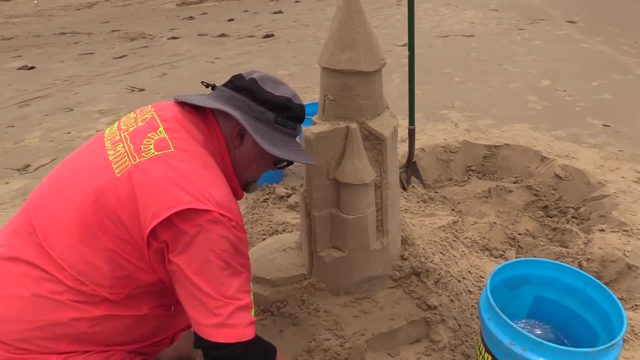 Um, you can flatten it out with your big spatula this time. The big spatula is just it just again, just gives you speed, but it also can clear a lot of sand very, very quickly, And we're trying to. 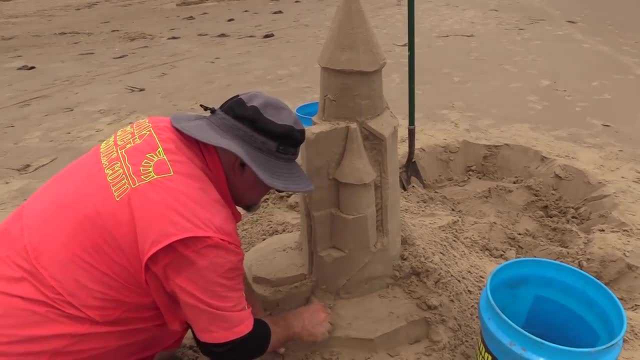 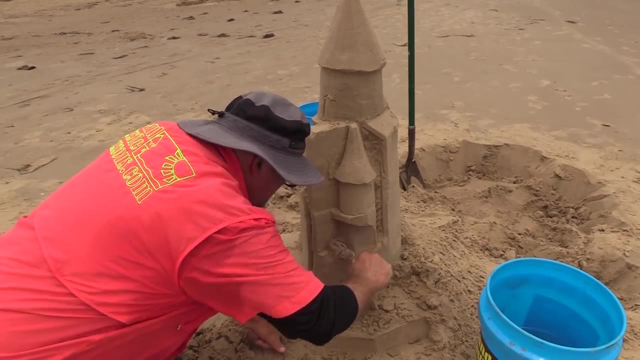 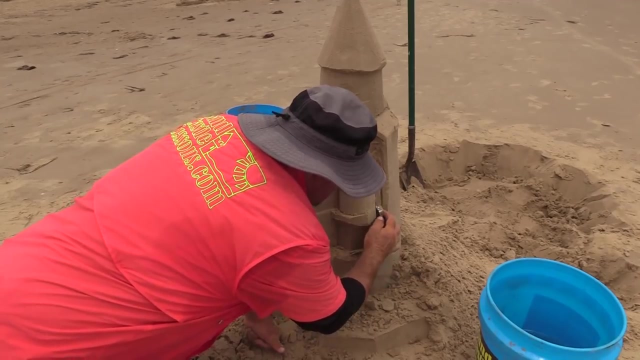 change out the shape of the base So then we can put another little staircase from this tower, which we're going to carve away, down to the other tower, um, or the other, um, little patio or, uh, courtyard or whatever you want to call it. Um, we're going down here and we're going to make 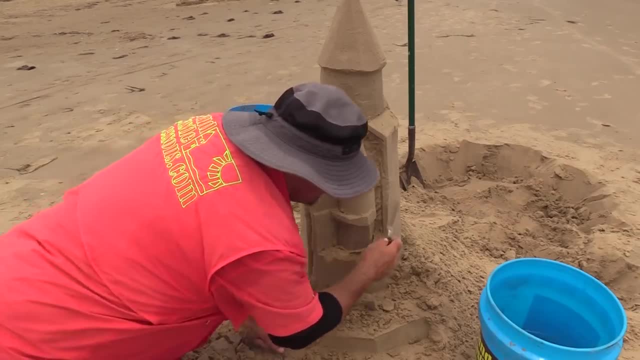 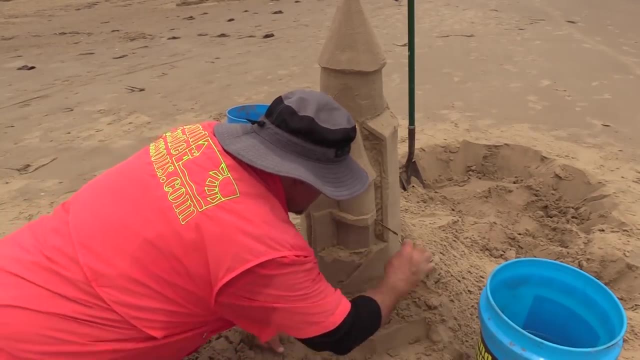 this nice and round And, uh, not particularly straight, Unfortunately, when you're doing this, one of the things you can't do is you must do, is you must get up and have a look at what you're doing, because you'll find that 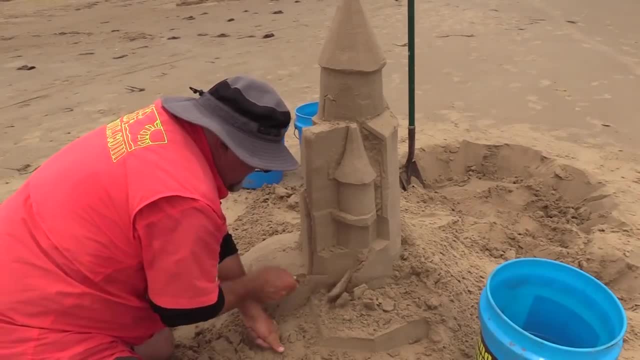 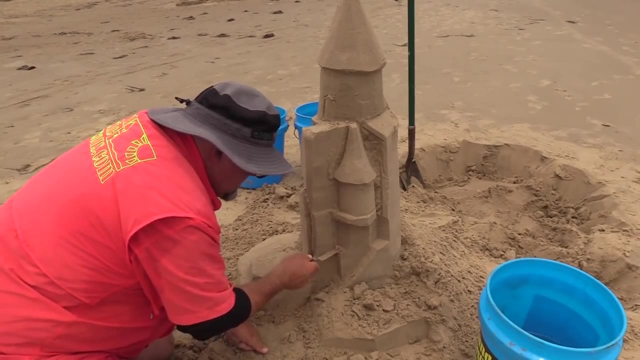 lines aren't straight and things you've done aren't right And uh. so it's important to get up and have a look, just like I didn't do in this video. So what I'm trying to do is separate this little building, make another set of steps and there we go. So we've made another set of steps that go. 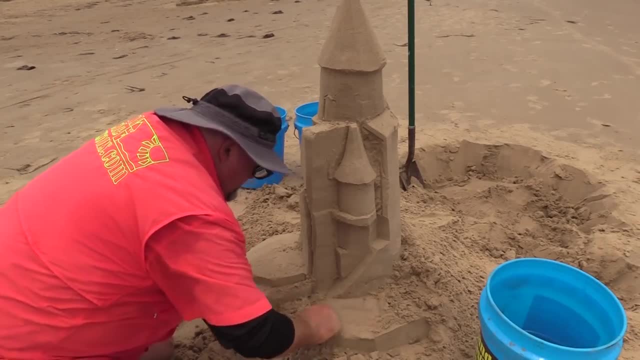 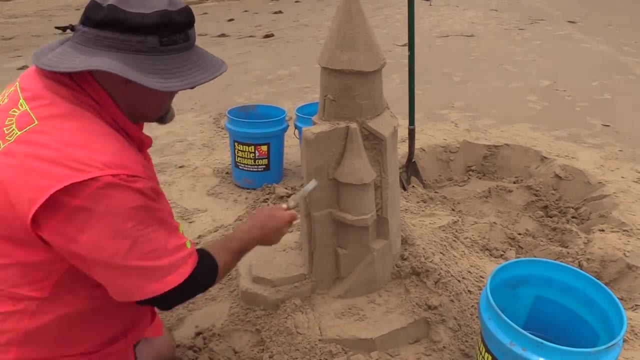 back onto this, but you can see how quickly we're moving down the castle. Obviously, we would be moving at the top before we did any of this stuff, but we're not doing that today, because we're showing you how to just use the spatula to get the shapes, Um, and it's very flexible, As I say. 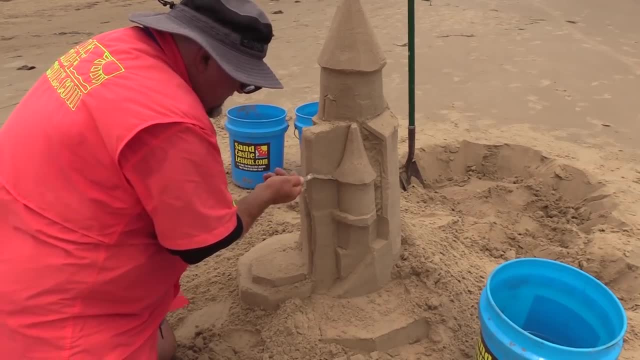 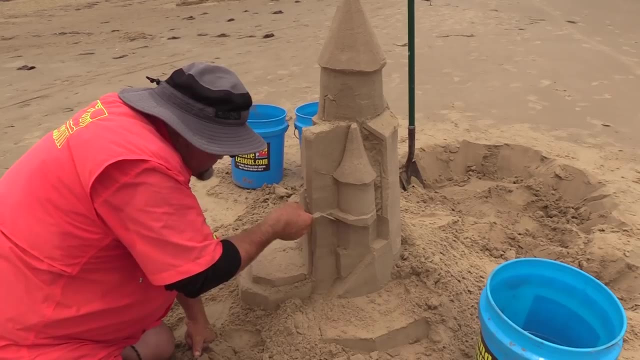 if you can use this tool, you can make anything. So we're going down there making the separating little building, making sure it's got a black line right into the side of it, And then and then trying to figure out how to get that tower to look straight, because it looks pretty ugly at the 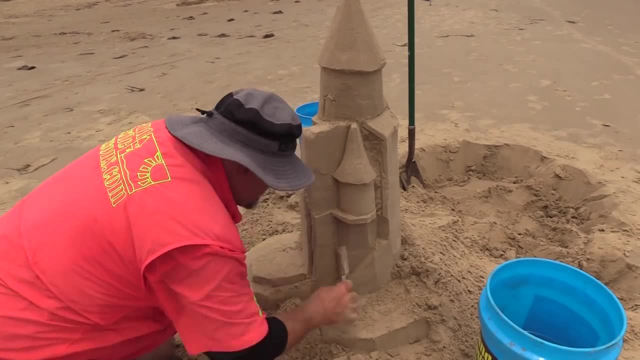 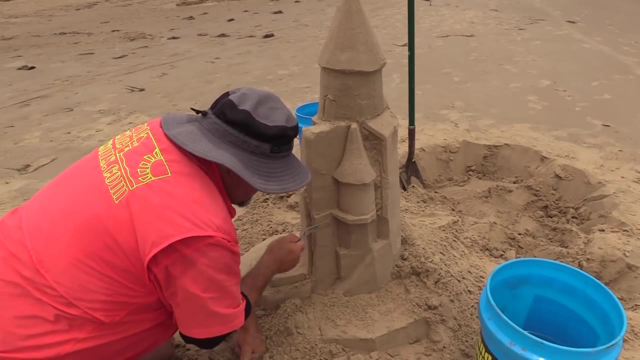 moment, There you go. That's looking a bit better. And then what we're going to do is put a- I think, a hexagon- hexagonal base underneath it. So we're changing the shape. It goes from a round tower to a hexagon, or a hexagon as they say in. 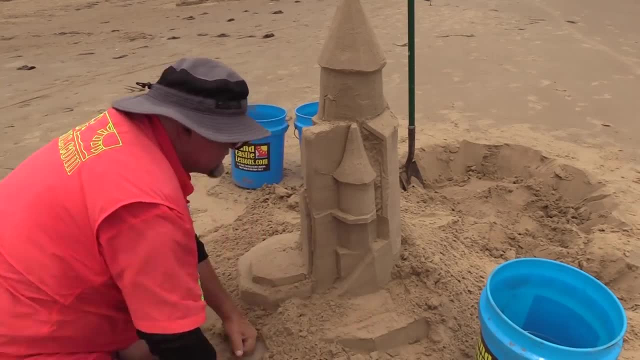 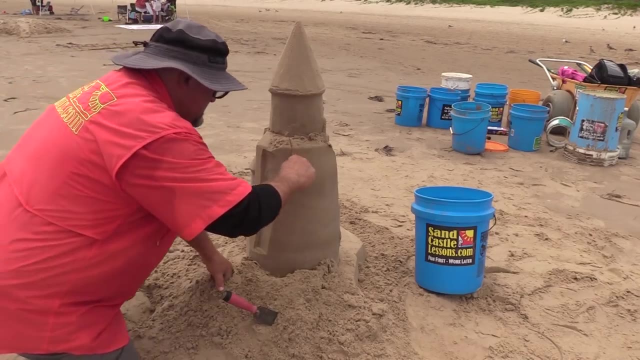 America. So, um, so, there we go, And that's how to change the shape. So then, we've done that on one side, We've still got a big old blob on the other side. So what do we do with that? Well, um, you. 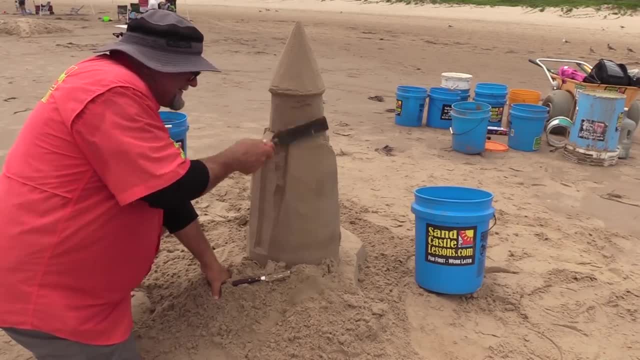 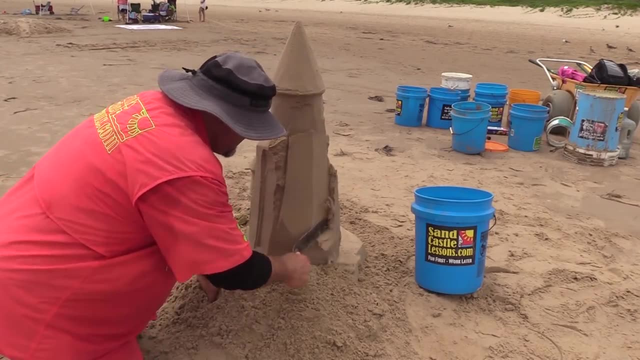 can use the big spatula just to take the side and we're going to make it into the tower all the way down. So we want a nice flared cone tower like a big cylinder, but a flared cylinder So like a stone, Um, and then. so we're going to use the big spatula so we can get a beautiful flat straight. 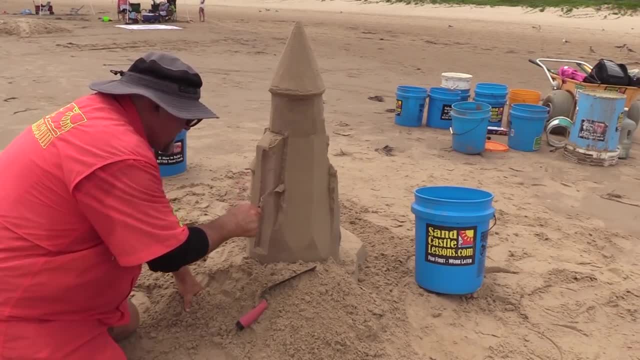 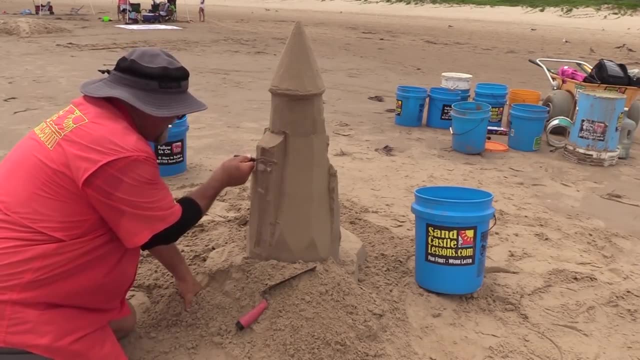 edge all the way down there. Then we cut the side of our building away. So we don't, we don't cut it away with the big one and do that. So what we're doing is making those buildings, the little buildings we put on, pop out from the main tower. Um, so people will say, well, how did you do that? 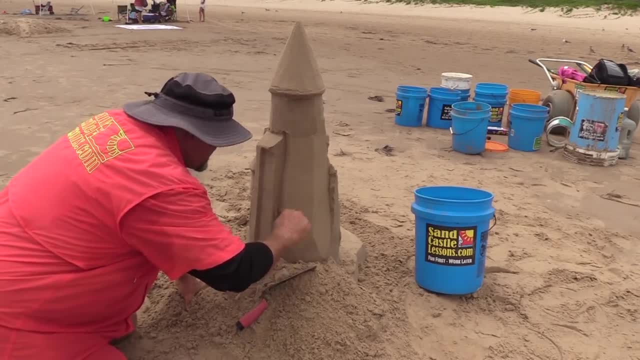 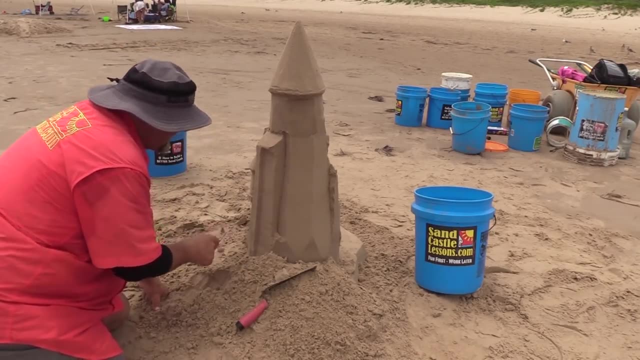 on the main one. You've got that building. Then this is the one pops right out the side of it. Well, this is how you do. you carve it. It's relief carved. Again. you carve it on the surface. So that's how we do that, And you can see we're using the little spatula. 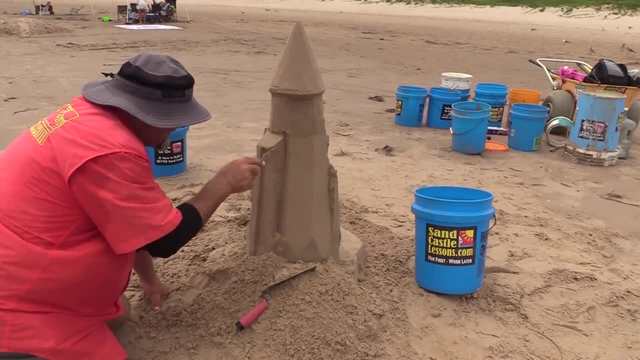 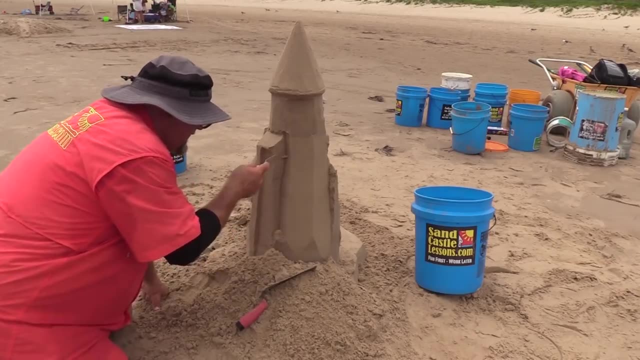 get a bit more control. You can see all the equipment we take to the beach in the background. We've got our cart and we've got the, obviously, the camera and all that stuff, but uh, we got, uh, lots of five gallon buckets and a two gallon and 10 gallon. Um, we have got a trash can as. 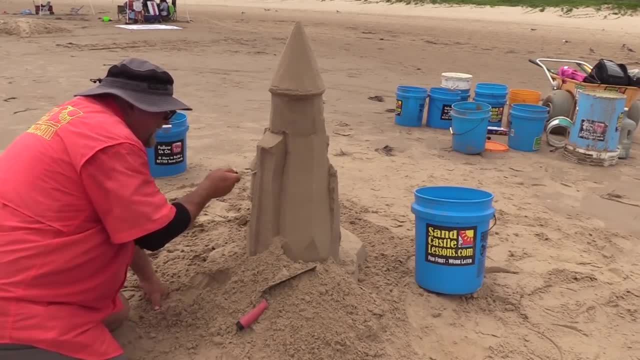 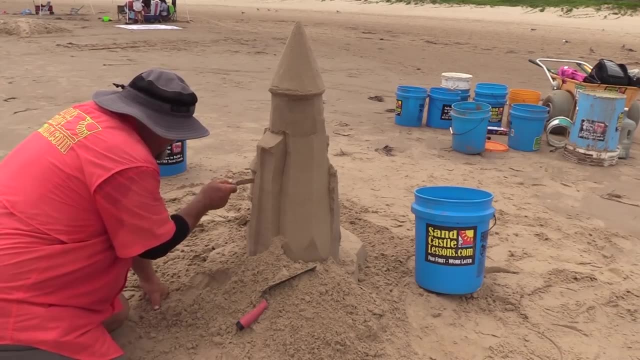 well, which is out of shot, but uh, we don't use that for this cause it's way too much Well for such a short video. So, um, we're doing that and I'm putting the other side of there now just to just to make sure that that's fitted, but uh, I should. 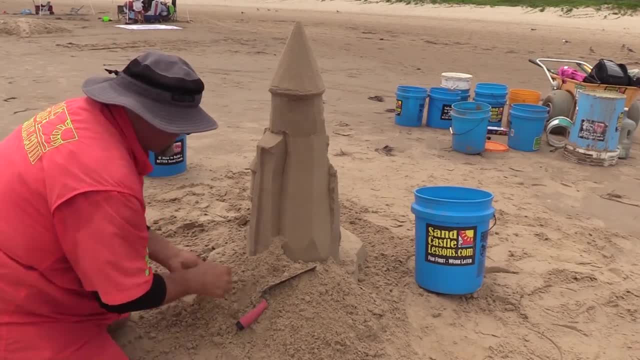 have done more on this side, really, but I, you get carried away in the moment, don't you? Yeah? So again, we're going to make, yes, again we're going to make a little moat I'm very good at. 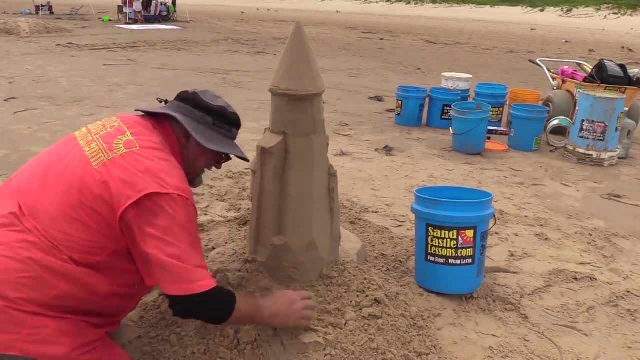 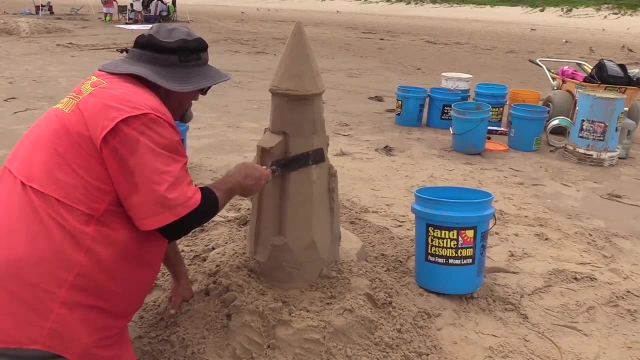 moat and, um, scratch this away again. We're reusing what we've already carved off, So we're not, uh, giving ourselves any, any extra stuff. Um and again, one of the things that it will do is it will enable us to join to this castle and make make it not look like a bucket. 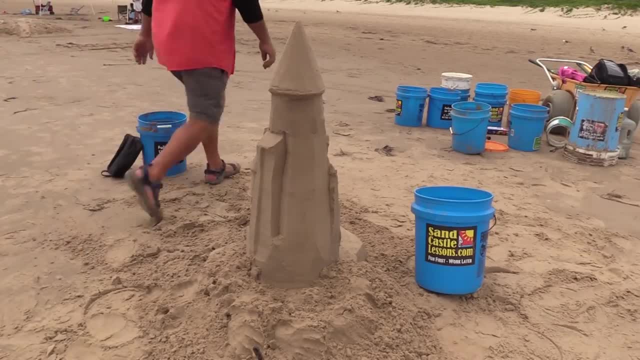 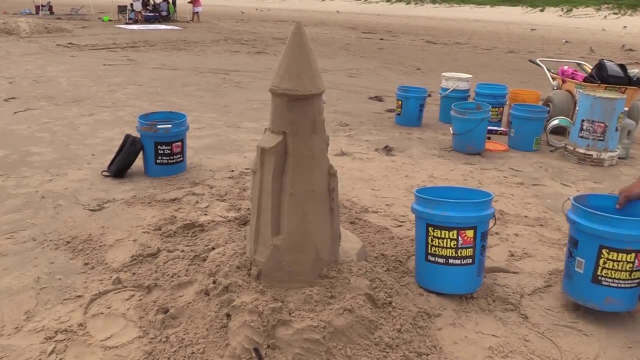 Um, so we're going to get the castle done there and then wander off and get more water. and uh, yes, Why didn't I use one next to me? No idea. Oh yes, I did, There is. I went and got an empty. 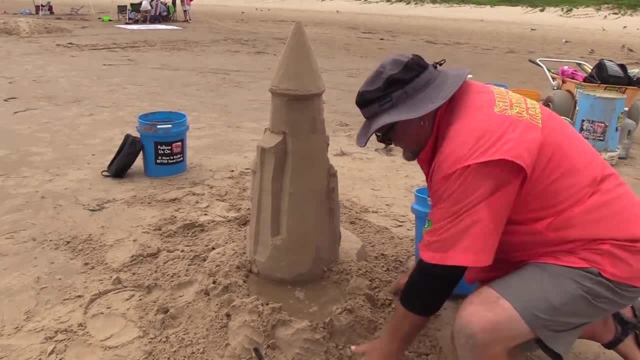 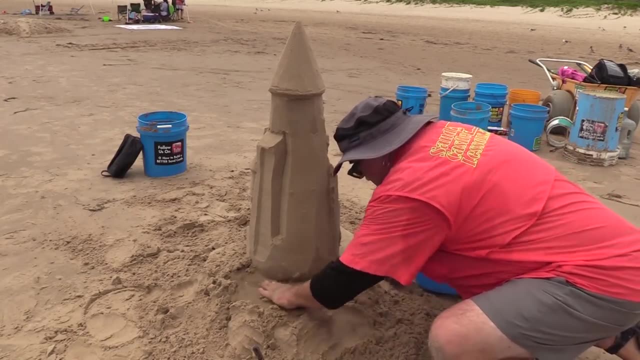 one and found out I had a full one, Nice. So we got that. We're going to, we're going to pull this up again and just fill it again and just get it nice and flat. Okay, Like that, Give it a bit of a pat. So if you pat it like that, what you're doing is you're just making. 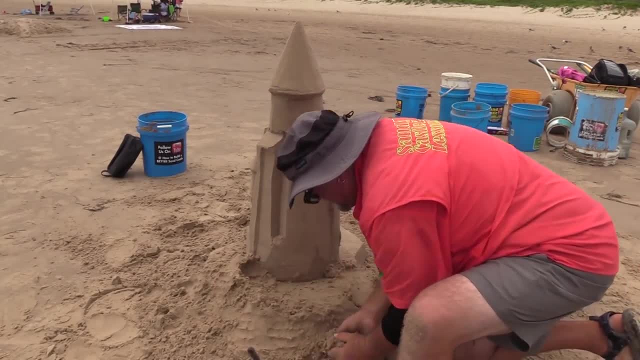 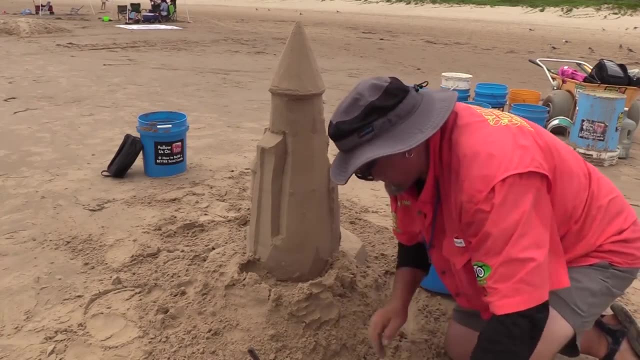 water travels through the side of it and we're making, we'll put the sides up again. If you want to go even higher, you just pack the soft sand and it's called soft packing. And, uh, if you're making something, you make it very quick by just packing the soft sand together. Then we fill it. 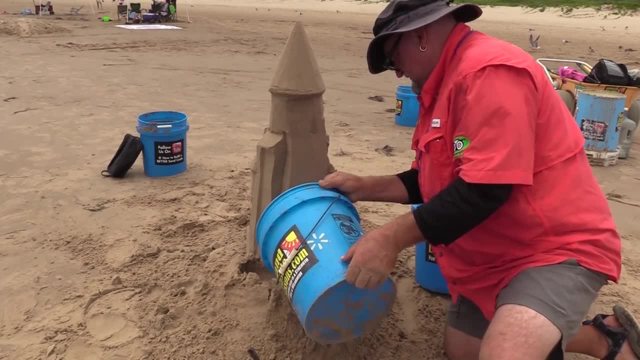 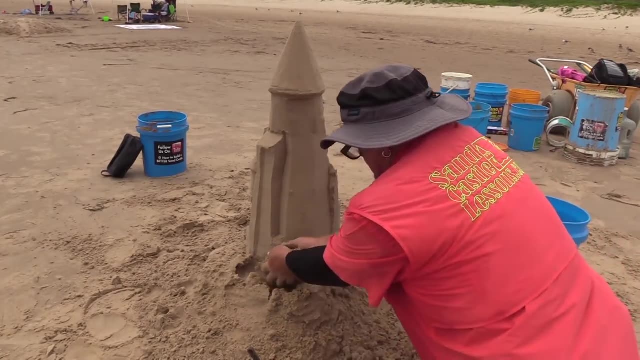 full of water again. Um, and yes, we use a staggering amount of water. If you haven't got water in a bucket at all times, well, and then we're just doing it there and filling that again, because we want to raise this side and we want to change the shape. We want to make this side have. 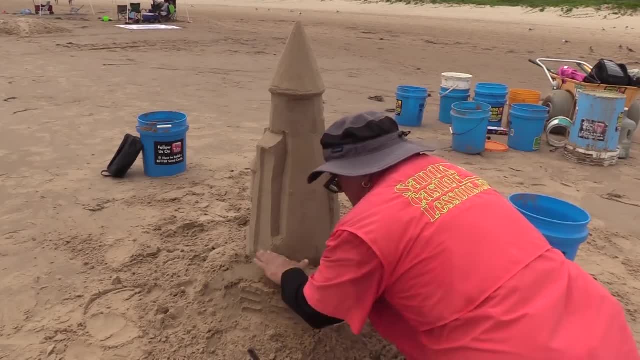 uh, be higher than the other Two sides. So we changed the perspective, the way it looks. also we changed the base So people can't tell it came out of a bucket. They're going: wow, that must've been enormous. How did they do? 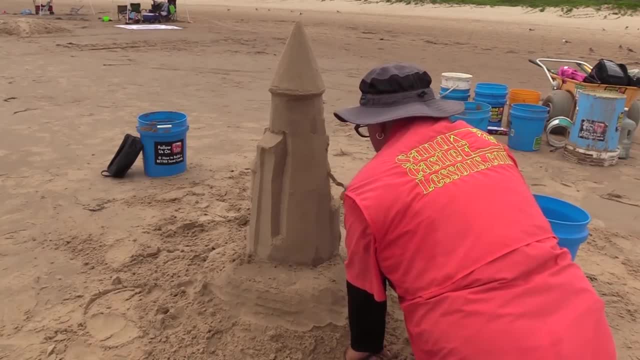 that Well, it's not enormous at all. What it is is: we didn't make it out of a bucket and, uh, we made it by hand, Um, but by we. by the time we finished, you shouldn't be able to tell we've. 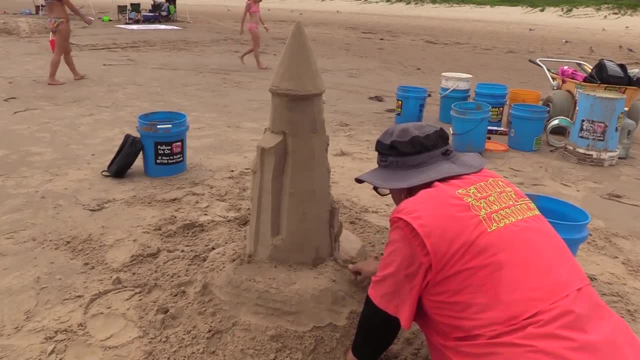 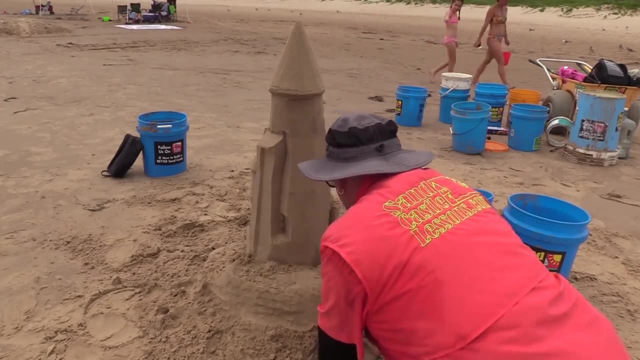 we've made it out of a bucket at all, because that will be a big fail, And we don't do that. We always have our fair share of fans and, uh, they come and look, um, and just watch us build, which is great. We love that. Um, I'm a public artist, so I don't 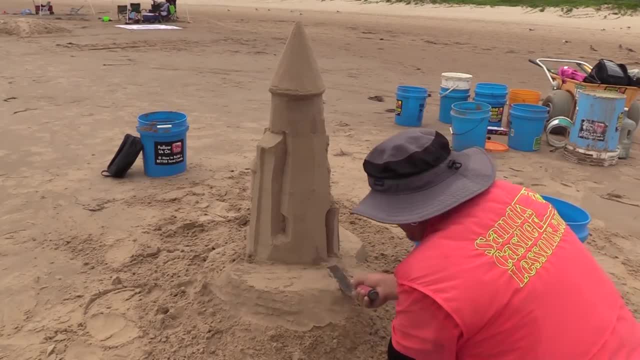 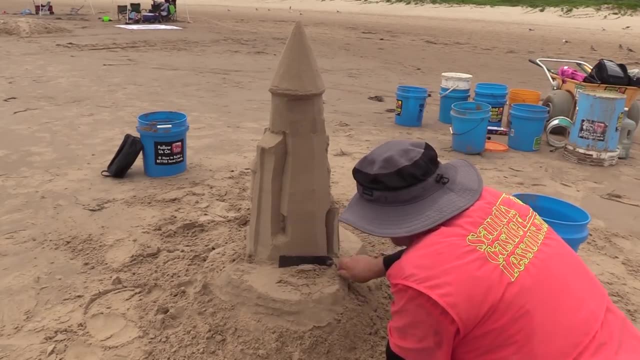 mind people watching me and asking me questions and stuff, because that's how they learn about what I do. So I also have to work. I'm a working artist. I don't have any other income. I I earn my income from my art and um, and you have to be ready to meet your public at any time. 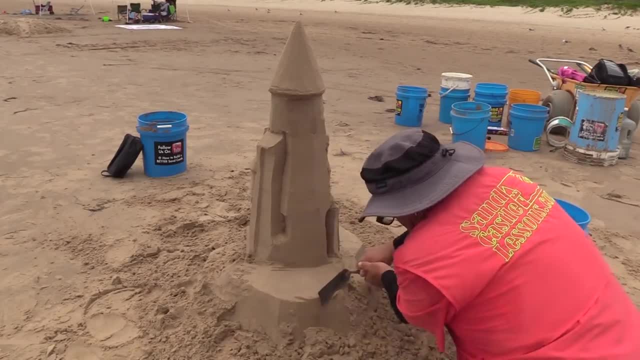 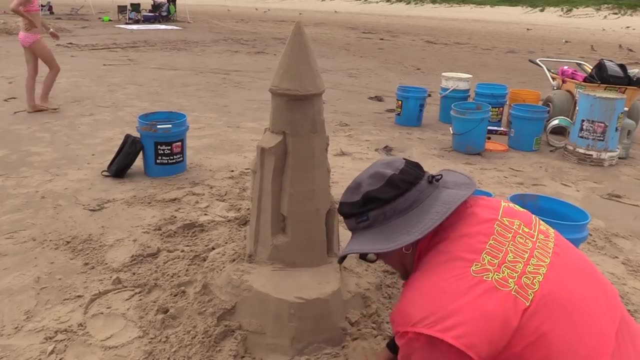 And they have to. they're always going to ask you questions, And if it's the same 20 questions every single day, who cares? I don't care, as long as they're happy, I'm happy. So so here we are, we've piled up that base and we're chopping it away, So we've got an even. 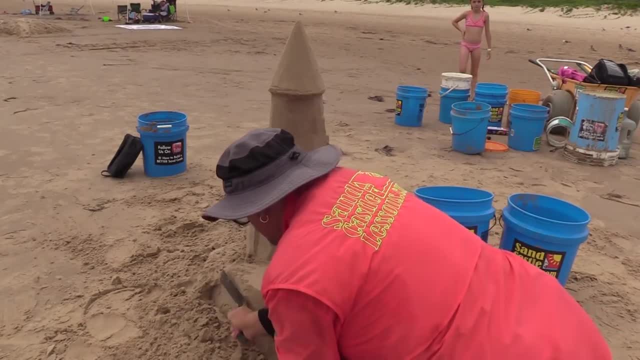 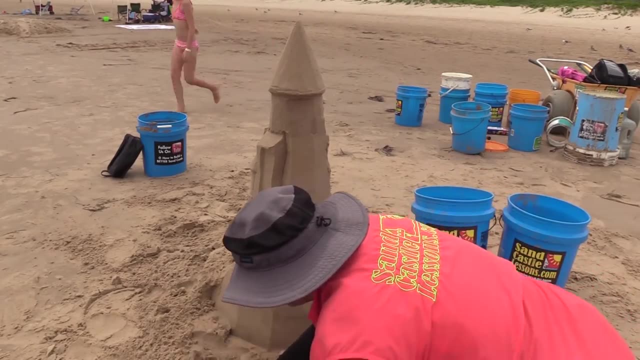 deeper side little tip: I learned off a, a lady called Suzanne Altamira from Florida, Daytona beach, Florida. He was a brilliant sand castle. uh, sand artist, sand sculptor- really, She doesn't do that Many castles. um, was that if you really haven't got any time? 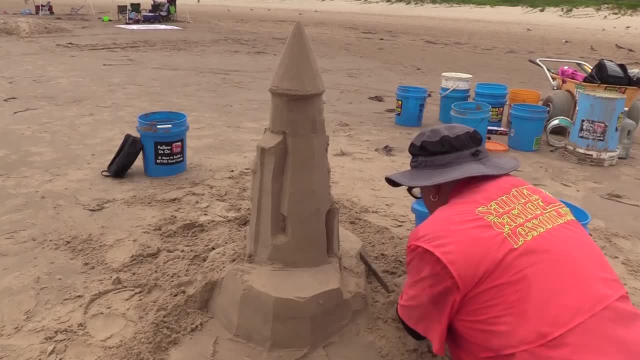 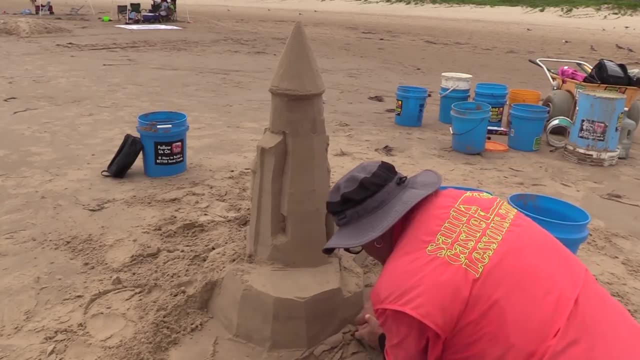 rather than trying to go up, you should go down at the same time. So when the judges came to come to you, look at your castle. if you've dug out something in front of it and made the stairs go all the way into the bottom and and whatever.